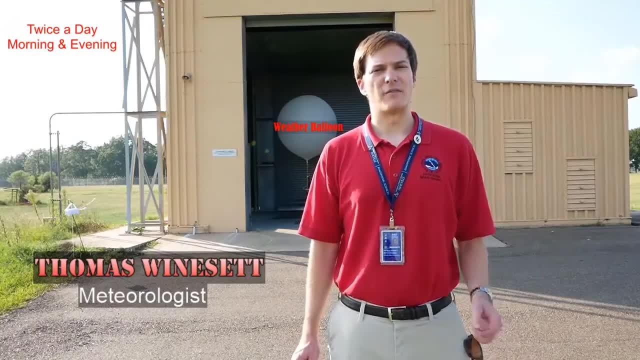 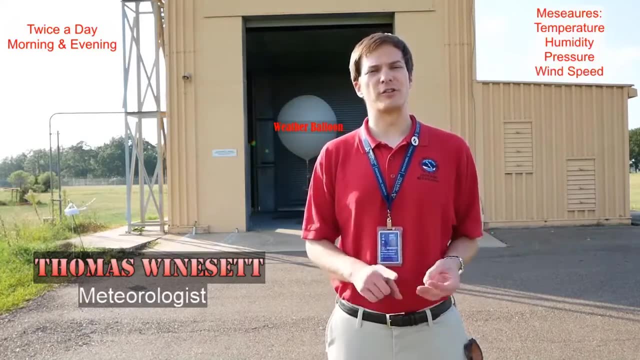 in the atmosphere, samples the atmosphere and provides valuable information back to us. So these balloons send data back once every second on the temperature, humidity, pressure and wind speed, And they go about 110,000 feet up in the air, which is 20 miles. 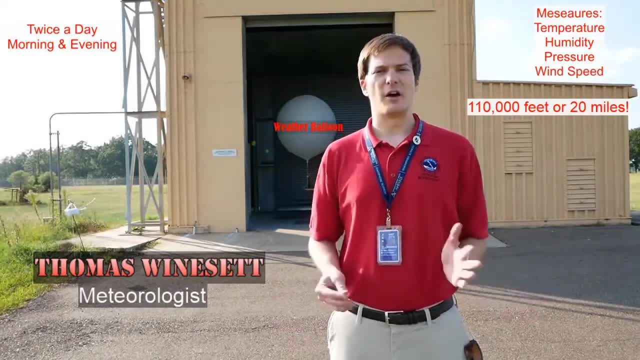 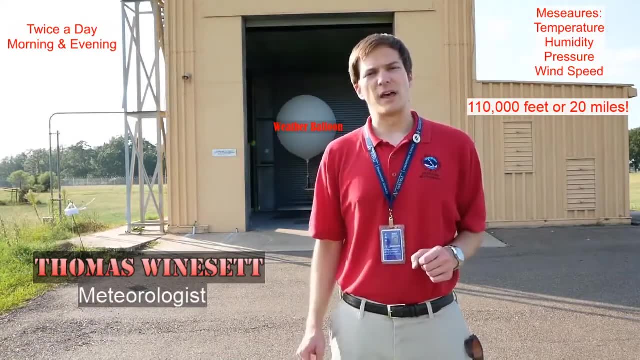 That's really high up in the atmosphere. That's higher than any planes fly. Planes only stop at about 30,000 feet or so, So they go pretty far up before they burst and come back down And we use that data to help make our forecast and we put it into some of the weather models. 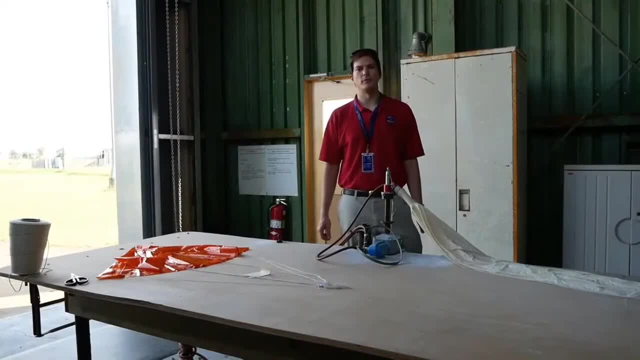 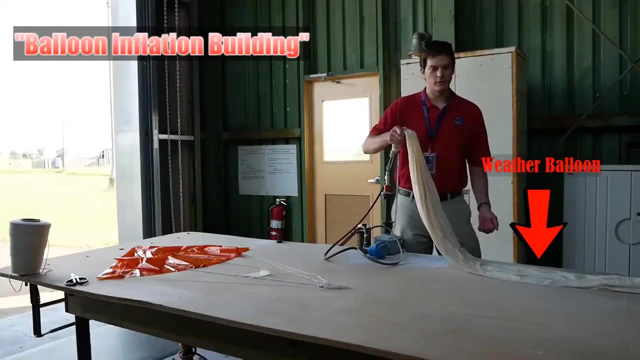 that we use as well. So now we are outside in our balloon inflation building and you could see here laid out on this table, we have a couple things. We have our weather balloon right here. It's this really long latex balloon. It's attached to this nozzle here And what we have is a. 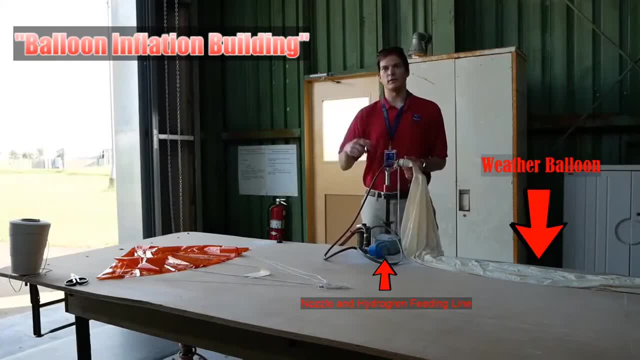 feeding line that's going to bring hydrogen into the balloon. And then here we have this feeding line. We're going to get that to this balloon And that's going to be the bottom from tanks in a separate room. through this line it's going to inflate the 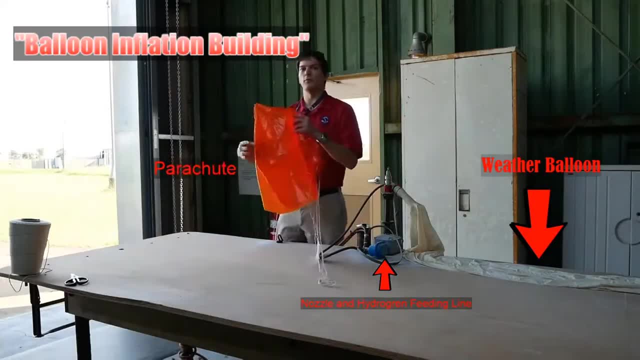 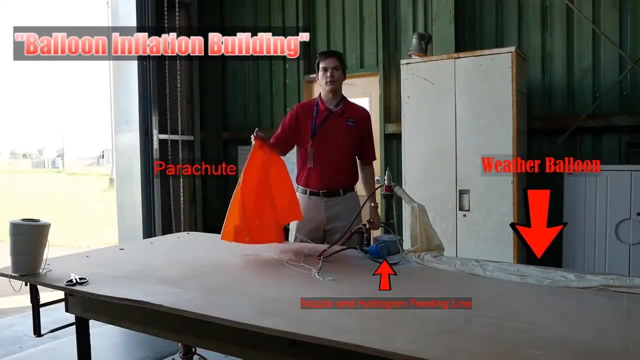 balloon for us. We also have a parachute here, so when the balloon bursts, once it gets higher up in the atmosphere, this parachute will help slow the fall, so it doesn't damage anything when it returns back to the surface of the earth. So now we're going to go ahead, turn on the hydrogen and start letting the balloon. 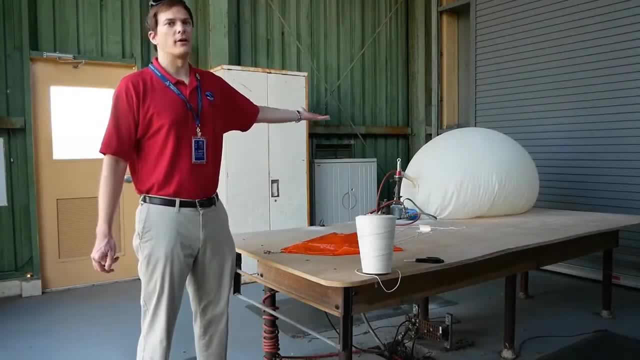 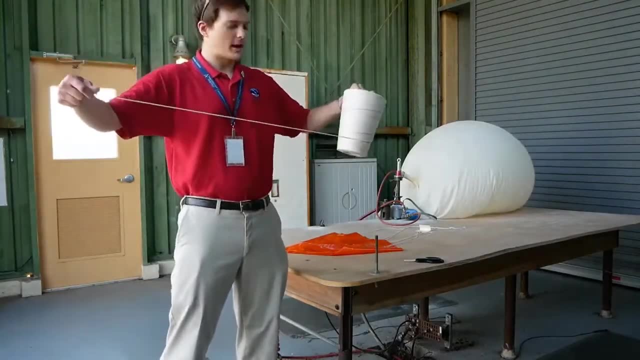 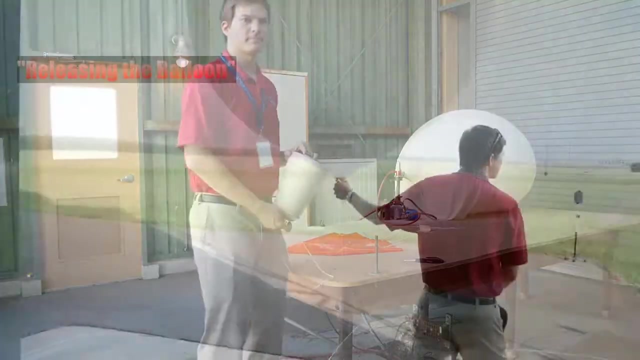 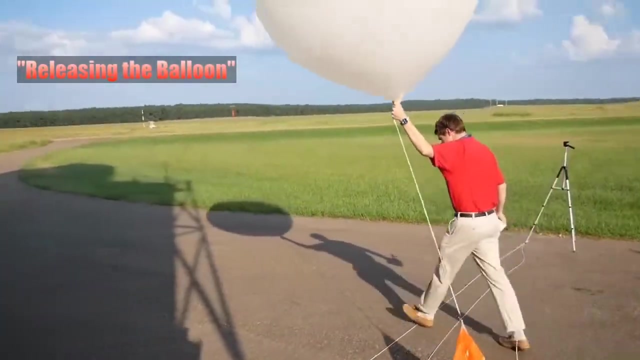 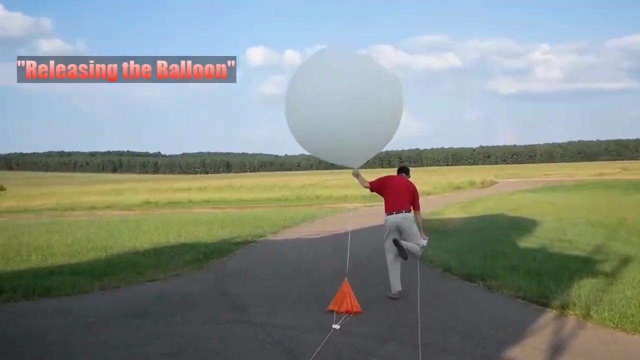 inflate. So while the balloon is inflating right over here in the background, we're going to take this stream and we're going to use this stream here to tie together the balloon to the parachute, to our Radiosonde instrumentation package, just sitting outside. Once the balloon is released, we head inside. 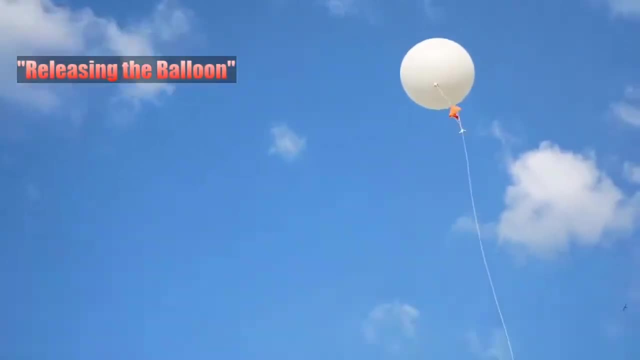 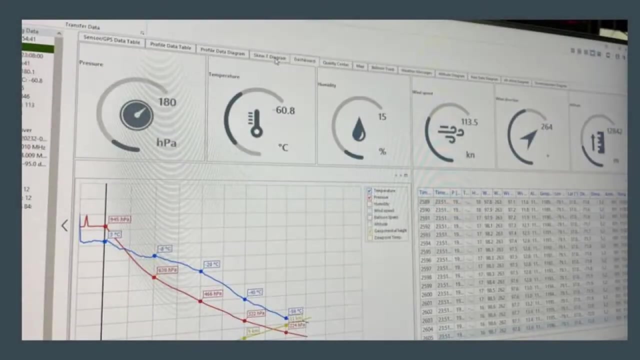 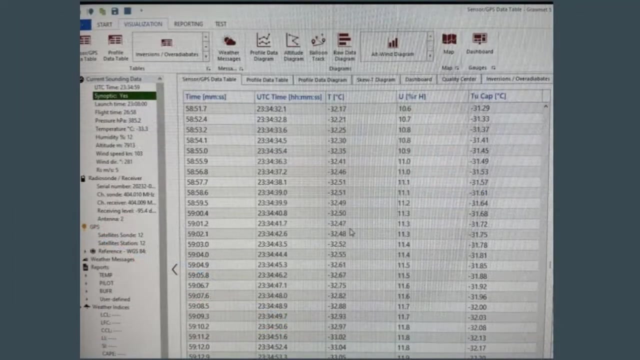 and we check on the data. We get pressure, temperature, wind, as well as humidity and wind direction as the balloon climbs through the atmosphere. We track that data here on our display, as well as the altitude as it climbs through the atmospheric column. Once again, we see the wind, as well as the humidity and 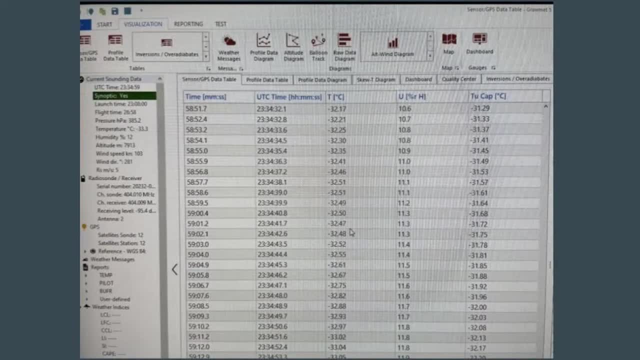 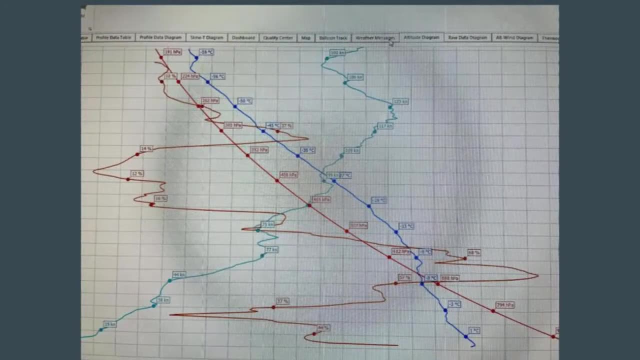 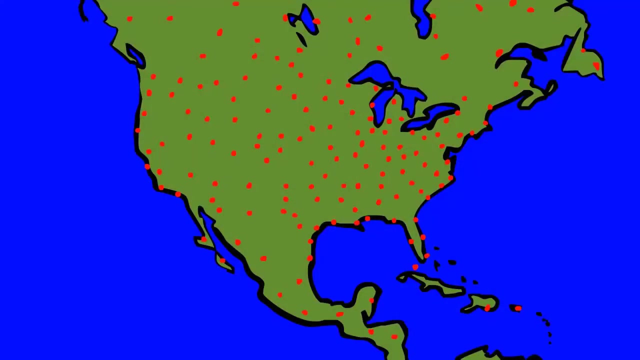 temperature. This is one way to look at it, a profile diagram of all of those features and, the most common way, the skew-t diagram, which tracks the cold as well as the warm and moist air In the atmosphere. 92 sites in the US launch weather balloons simultaneously.